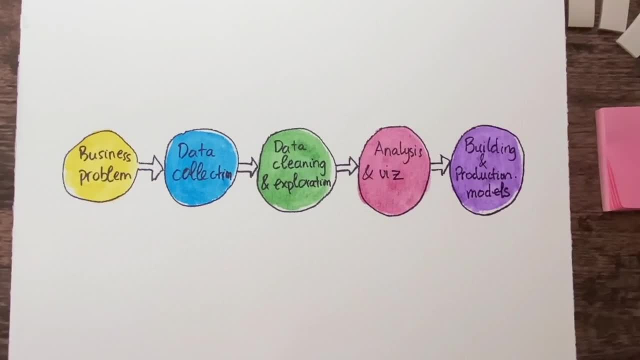 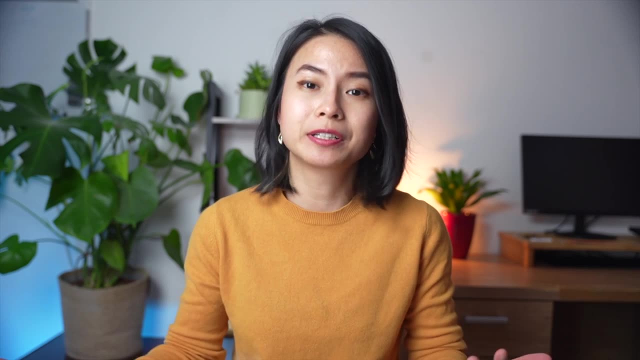 Model deployment is one of the important steps in the data science pipeline. It's getting more attention of businesses and data science teams nowadays as data science and machine learning fields become more mature. However, it's been found that up to 87% of data science projects 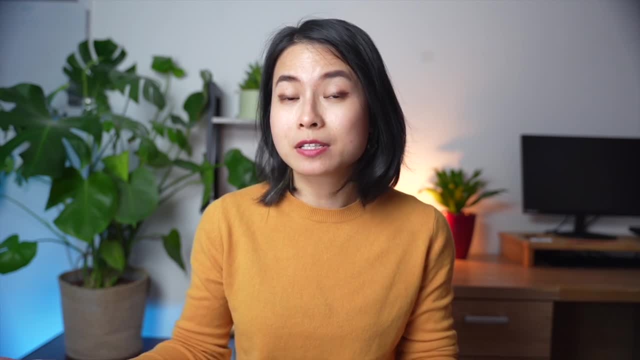 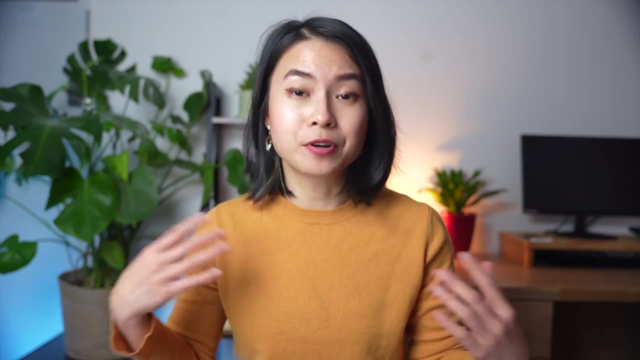 never make it into production. That means that most Jupyter notebooks created by data scientists are put on shelves to collect dust and never get used. It's getting easier than ever to create a predictive machine learning model, But in fact, many data science teams struggle to bring a model. 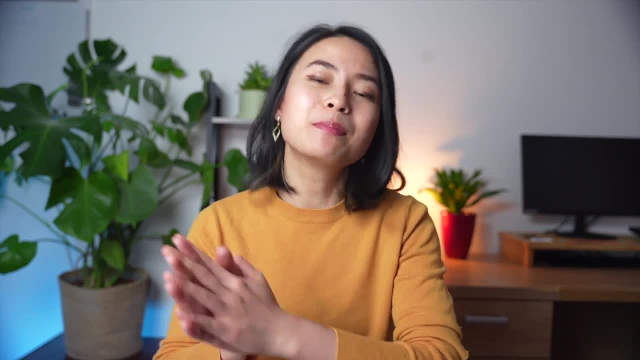 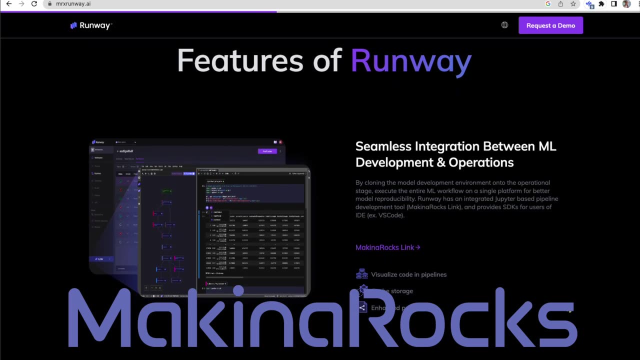 to real life to create actual impact. So in today's video, I'll be showing you how to deploy a machine learning model using Runway, an enterprise machine learning ops platform developed by Makina Rocks, who has kindly sponsored this video. This video is also an: 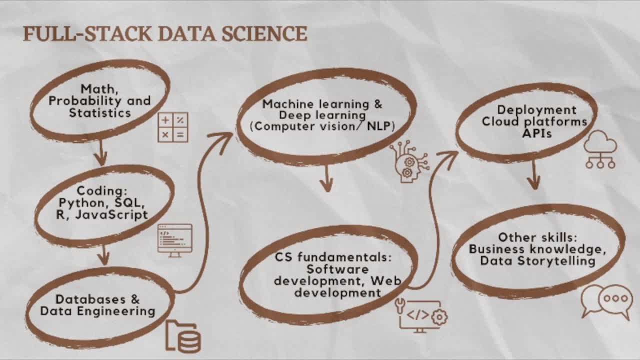 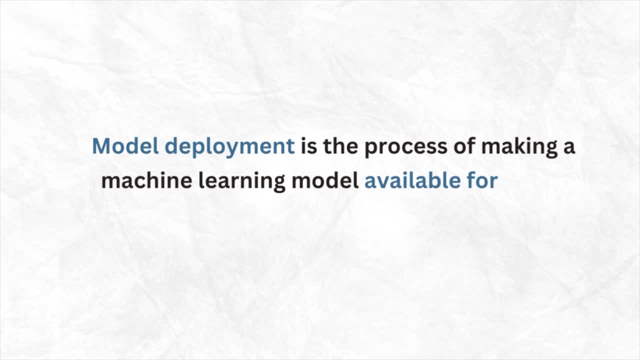 extension of an earlier video I made about how to learn full stack data science, So feel free to check it out here for more detail If you're not yet familiar with it. model deployment is the process of making a model. It's a process of making a model. It's a process of making a model. 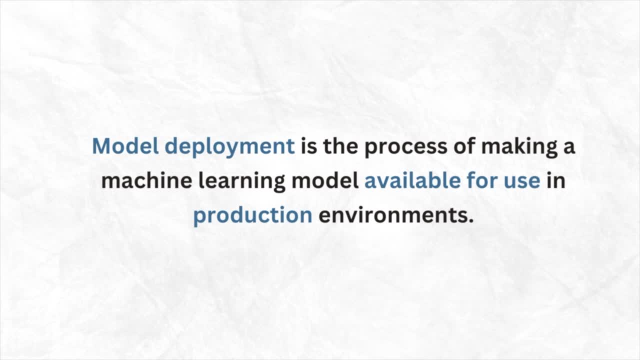 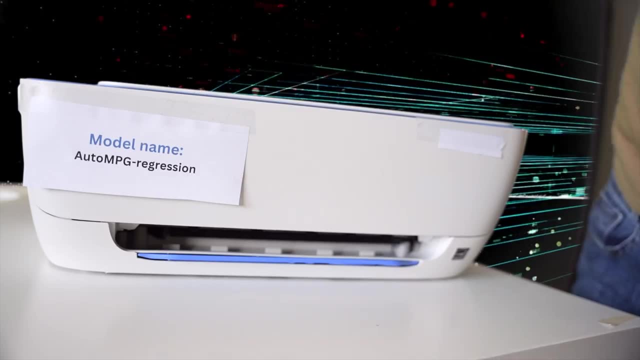 It's a process of making a machine learning model available for use in production environments. So what does it actually mean? It means to take a machine learning model that has been trained on a dataset, package it and store it in a format that can be used by the deployment platform. you. 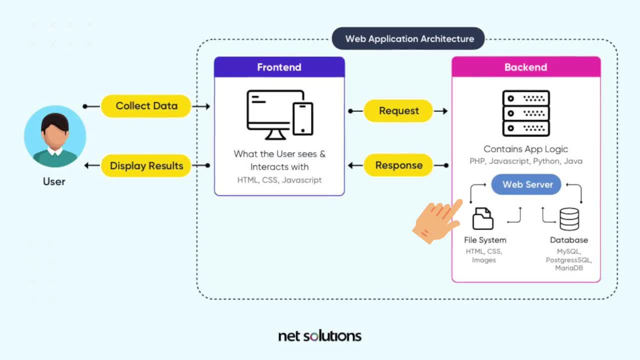 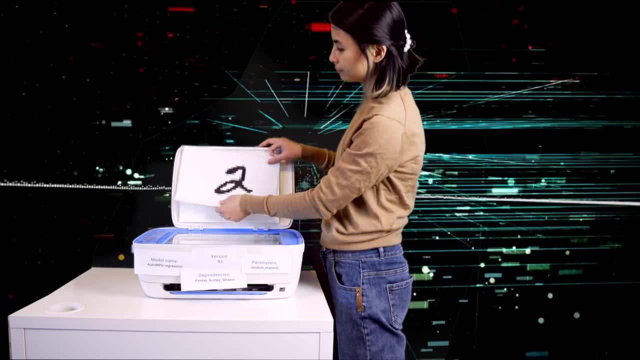 are using, Then we integrate this model into an application, say a web app or a system that can be used by end users. Users or other stakeholders can now interact with the model, For example, give the model some data input and get back the model output. This is, of course. 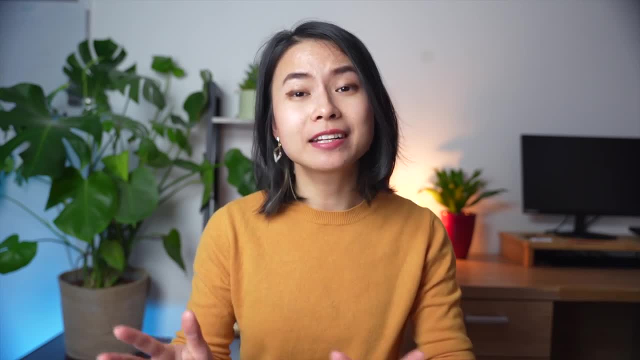 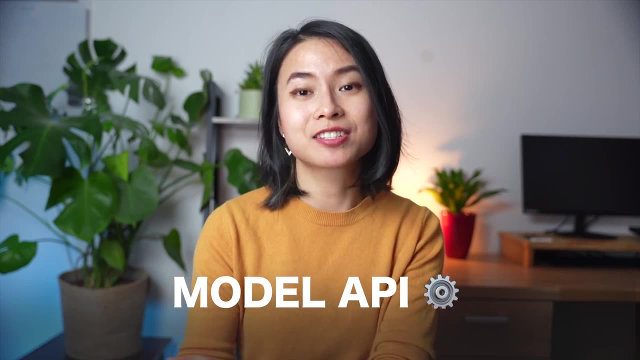 a metaphor to help you easily understand the concept. In reality, you don't need to physically interact with the model, but you can do it remotely through the model API. We'll see how this looks like in a bit. There are essentially three steps in model deployment. Firstly, we need 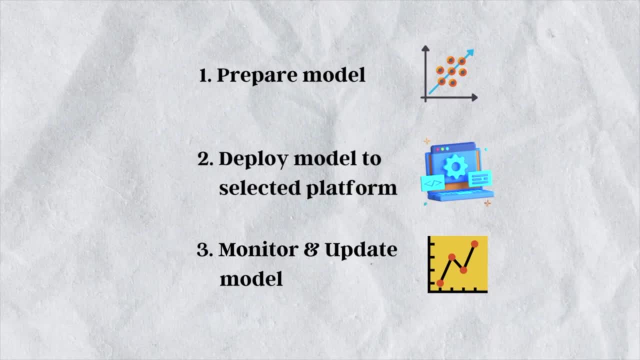 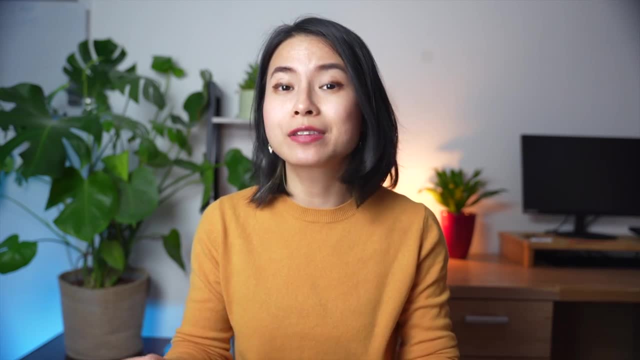 to prepare the model. Secondly, we deploy the model to the selected deployment platform. And thirdly, monitor and update the model. We need to monitor the model performance to ensure that it is performing as expected. Over time, the model performance will slow down and the model performance 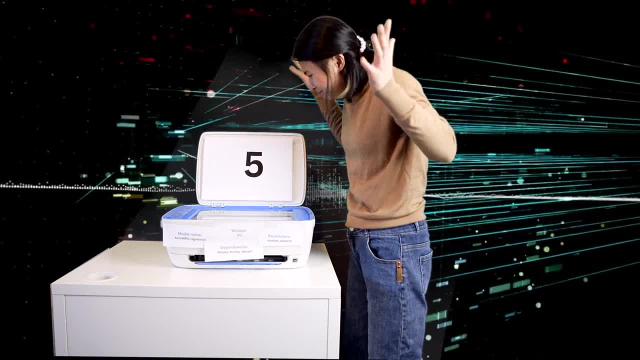 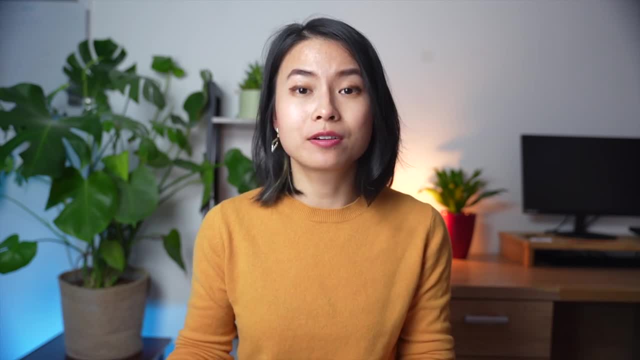 start to deteriorate as data is changed or there is new economic situation or there are new customer behaviors or preferences. When that happens, we need to debug the model, investigate what goes wrong and then the model should be retrained and redeployed. It's good to mention that in big 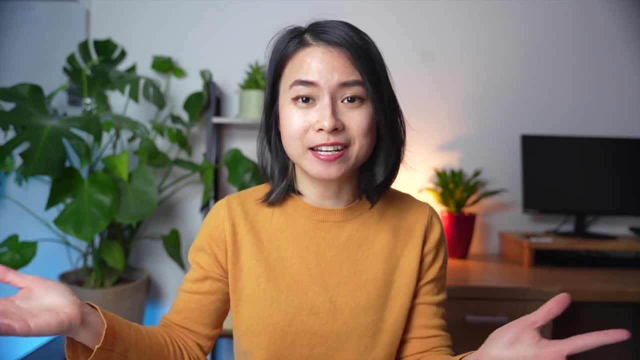 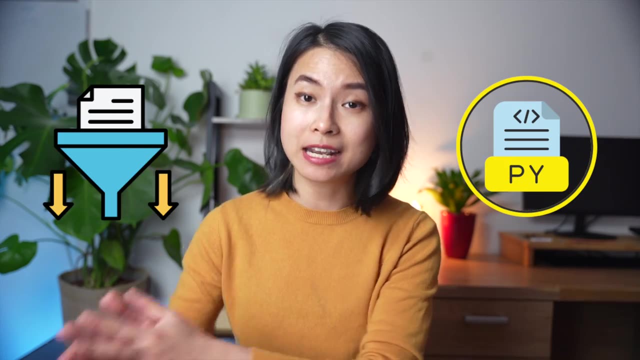 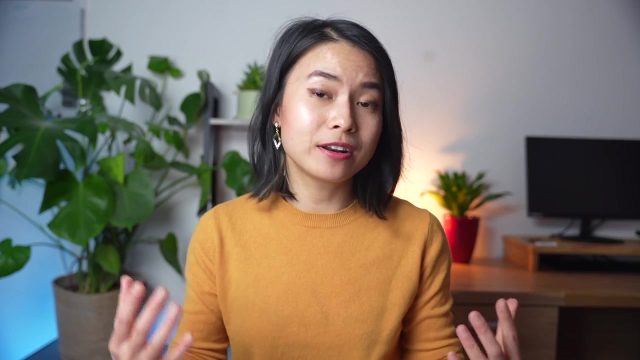 companies, they usually have a whole team of machine learning engineers to take care of productionalizing machine learning models using the model code created by data scientists and the data pipeline created by data engineers. In reality, though, in many smaller or less tech oriented companies, this is often not the case, and that's part of the reason why the model would stay. 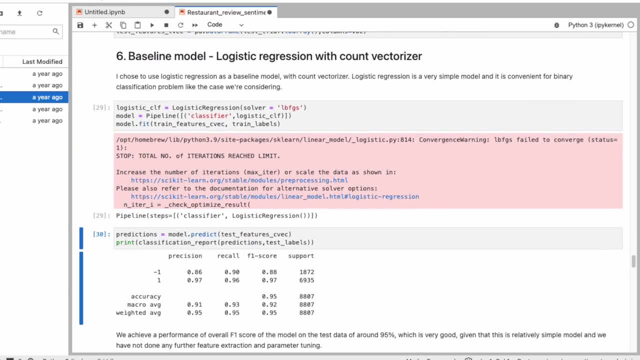 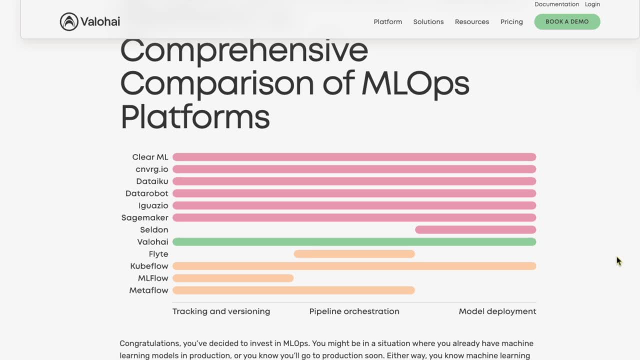 forever as prototypes in Jupyter notebooks and never get used. There are many machine learning ops platforms in the market for deploying models. They are complex products and it's tricky to compare them in detail. Now let me walk you through how to use Runway by Merkino-Rox. It's a very 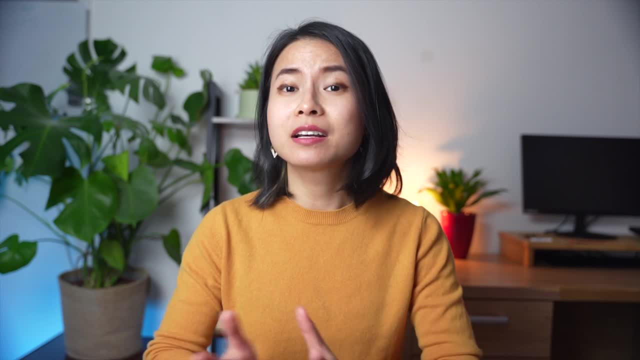 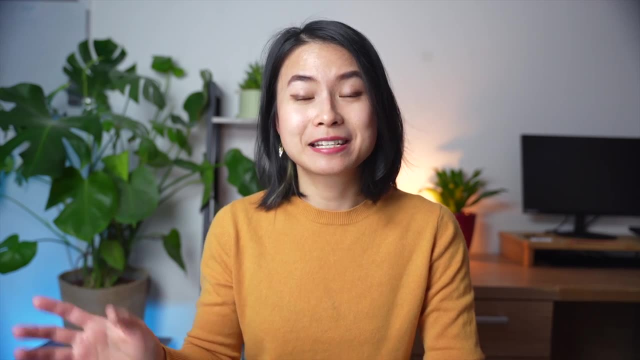 simple and easy to use machine learning ops platform. I find it a very useful and easy to use machine learning ops platform. It's a bit more native and friendly to data scientists because it can work directly with Jupyter notebooks, but with a clever twist to avoid the limitations of notebooks, which I'll 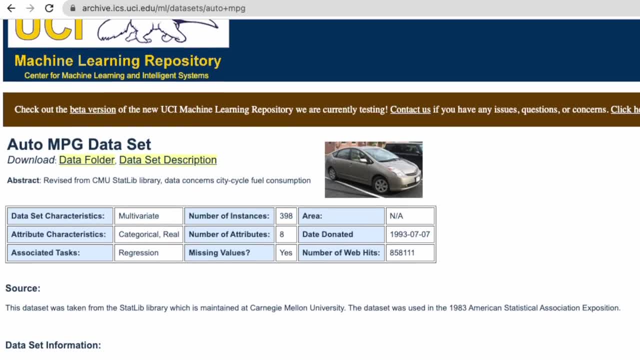 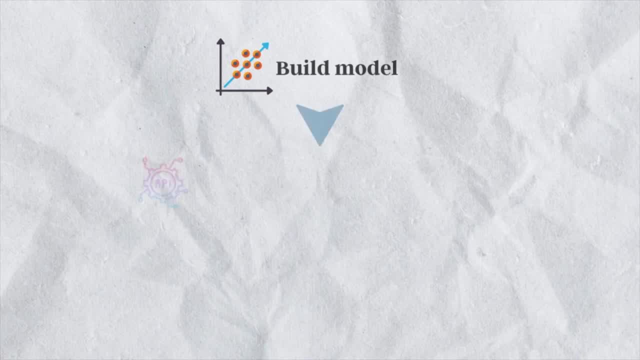 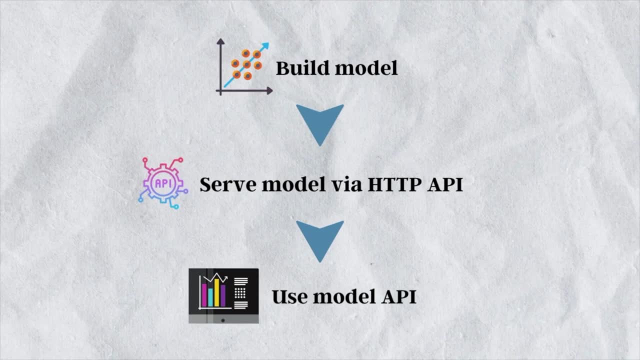 show you in a bit. In this stylized example, we'll be using the AutoMPG dataset to build a regression model to predict the miles per gallon of a car. We then learn how to solve the model via the HTTP API and learn how to interact with the model to get the predictions for a given data. 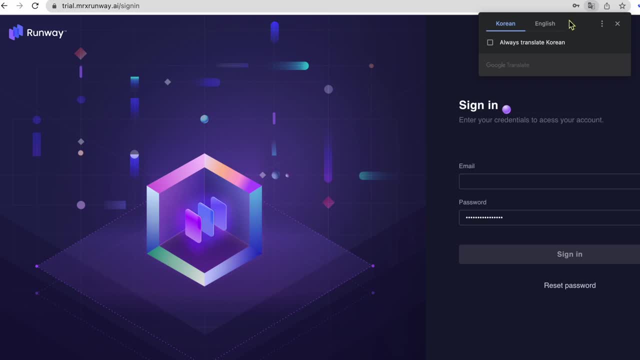 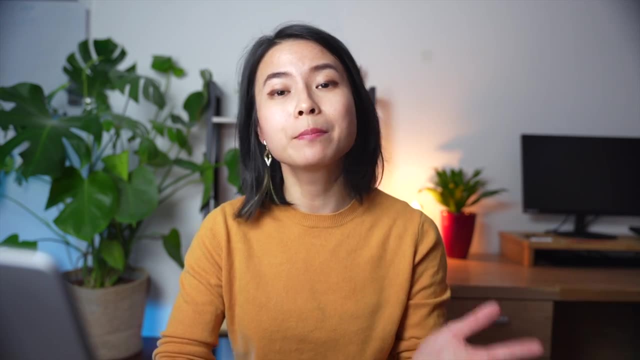 input. All right, let's go to the Runway main page And I'll sign in using my credentials. Currently, Runway is an enterprise solution, So if you want to try out the platform within your company, you can contact them for a free trial. They are very. 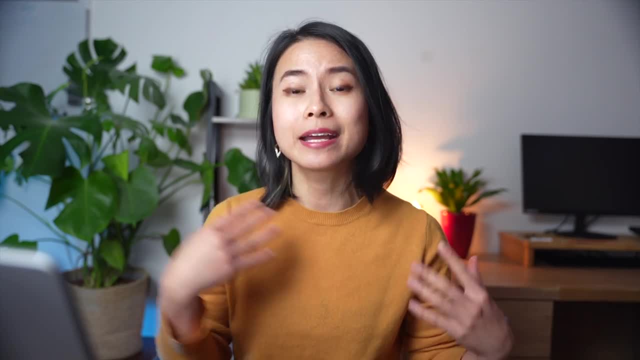 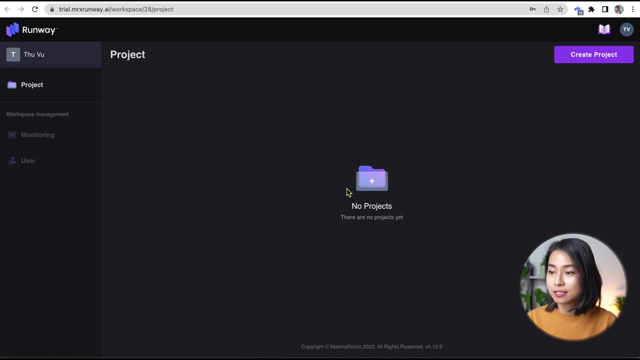 very nice people to work with. They are also now working on making the platform available for individual users, So let's keep an eye on that. After we sign in the platform, we see here: this is the Runway service console, And now we can go ahead and create a new project. And here: 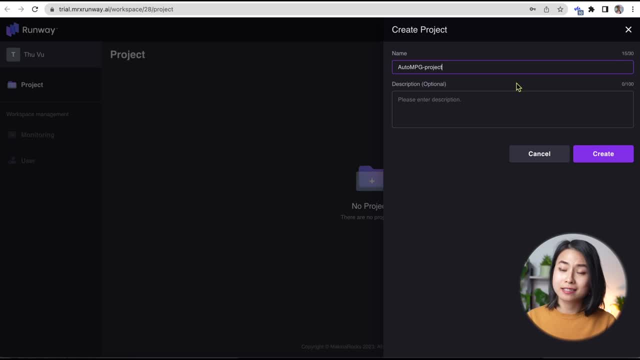 we can enter the name of the project, And I call this project AutoMPG. We can optionally put some description of the project here, So let's go ahead and click on Create. Now that we have the project over here, let's click on it to enter the detail page of our 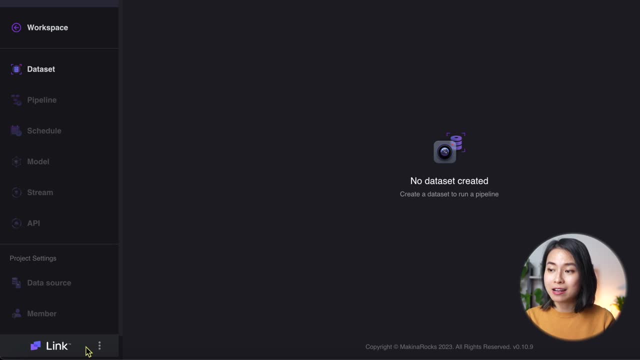 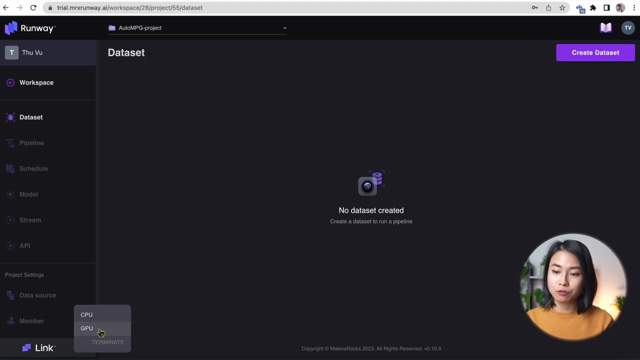 project At the bottom left of the screen you can see that there's a link area over here And if you click on the three dot button, you can select either the CPU or the GPU for our project. And I'll use the CPU for now because this is a very small project, As the computer finished setting up. 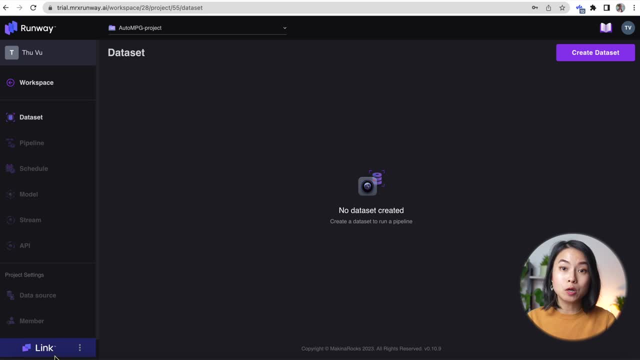 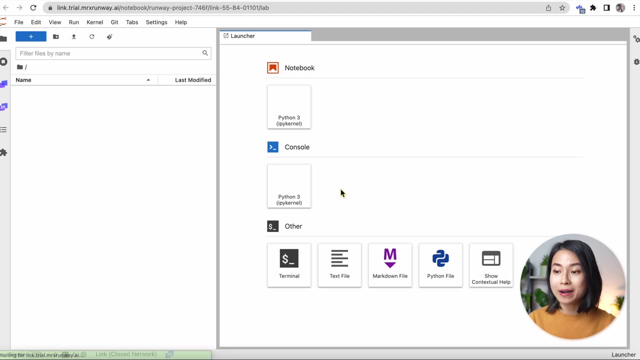 you can see that the link area now has turned to the blue color. Let's click on the link area And now we'll be directed to a new web page that's opened up, And this is the model development environment, which is essentially the familiar JupyterLab environment, But this is hosted. 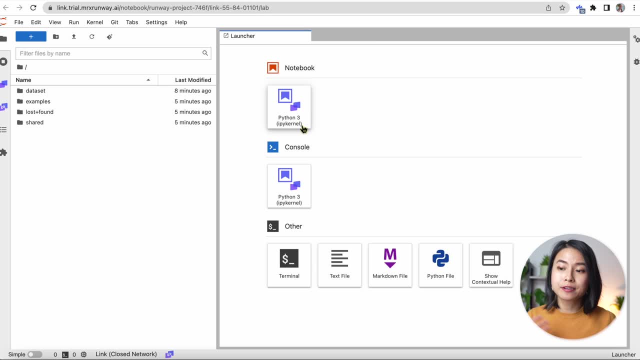 remotely on the Runway platform. You can choose to either create a brand new Jupyter notebook over here or you can also upload a Jupyter notebook that you already have. In this case, I have already created a Jupyter notebook for the model. 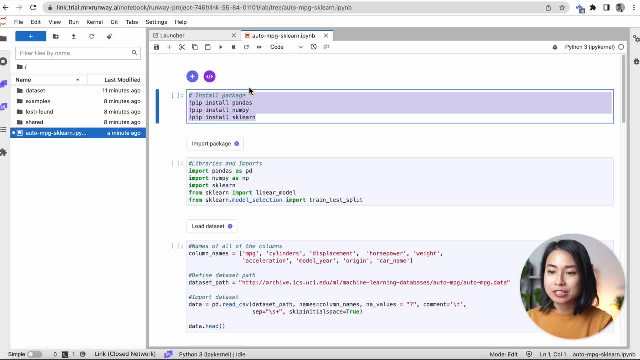 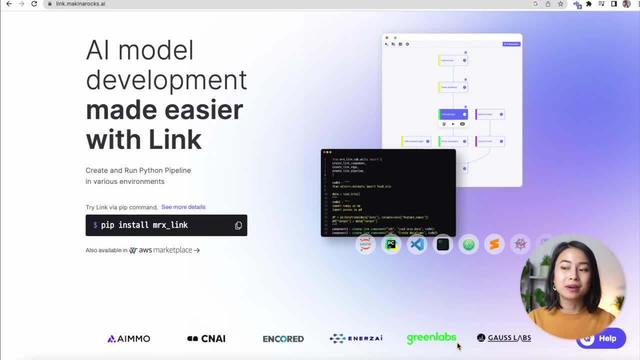 Let's now take a look at the model. I installed some necessary packages here. it's good to mention that this notebook makes use of the link extension, which is developed also by Makina Rocks. The idea of this extension is that it allows us to create a pipeline on top. 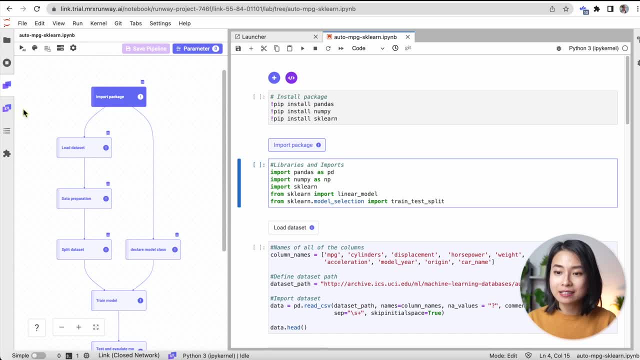 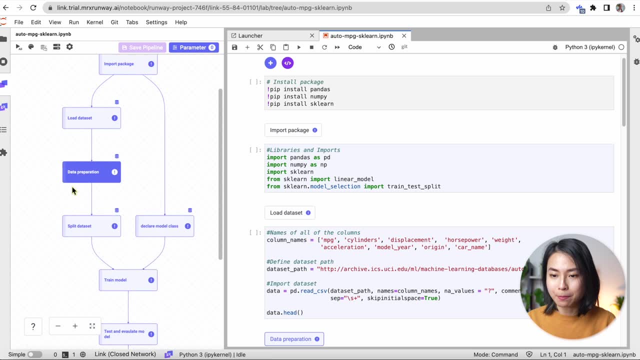 of the existing code cells. To explain what that means, if you click on the link tab over here you can see a diagram showing the whole pipeline of this model. So if I zoom it in a little bit more, each of these components on this pipeline corresponds. 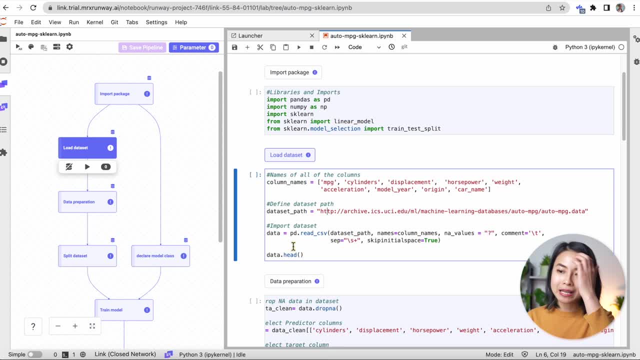 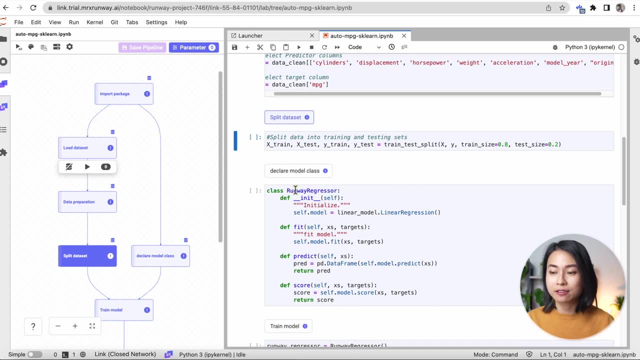 to one code cell in this Jupyter Notebook. It's all up to us how we design this pipeline, how the components are ordered and how they are connected to each other. For example, this cell or component LoadDataSet has the parent component ImportPackages. 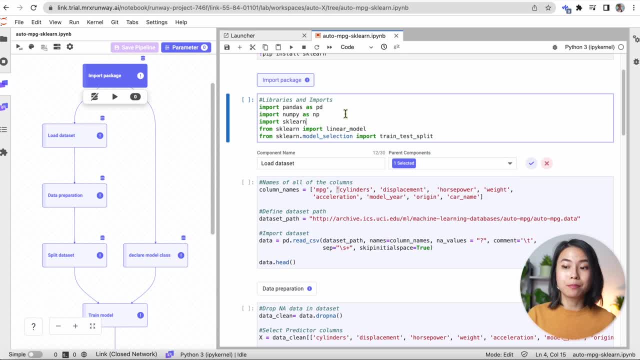 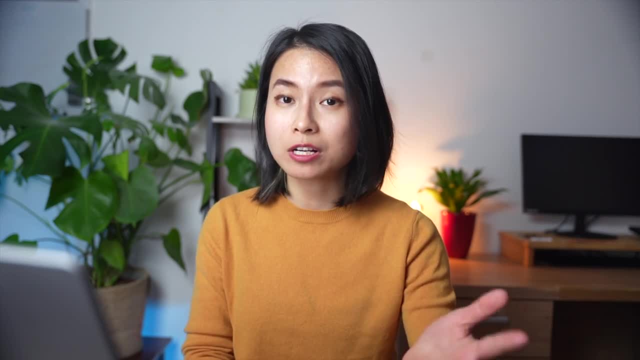 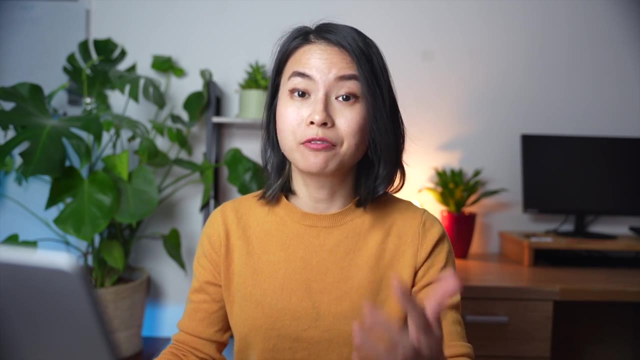 which means that the component is only run after we import the packages. So the purpose of this link extension is to help everyone easily understand the dependency structure of the code cells and the execution order of the cells. This can make projects built in Jupyter Notebook more production-ready. 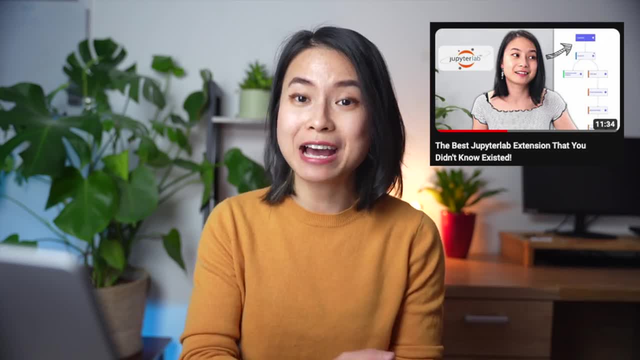 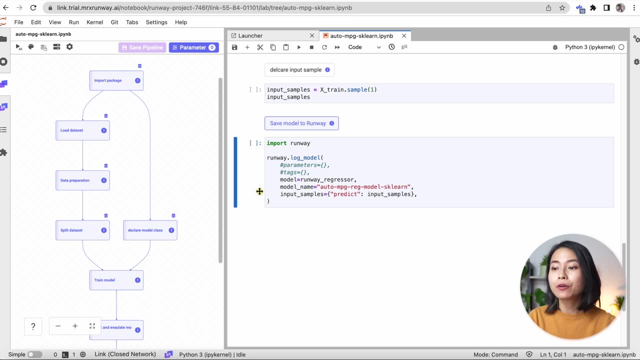 I've made a whole video on the link extension a while ago on my channel, so feel free to check it out if you want to learn more, If you want to add a new component into this pipeline. it's also very simple. Let's say we have a cell to print something like HelloDataNodes. 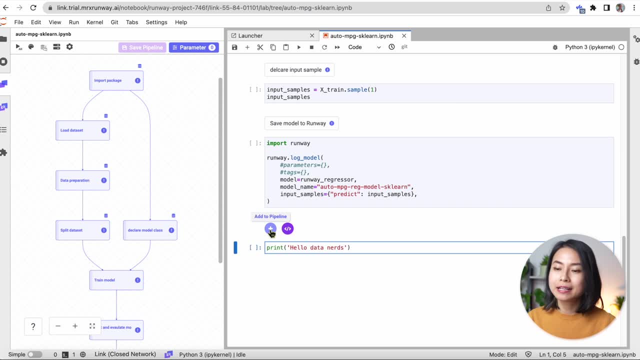 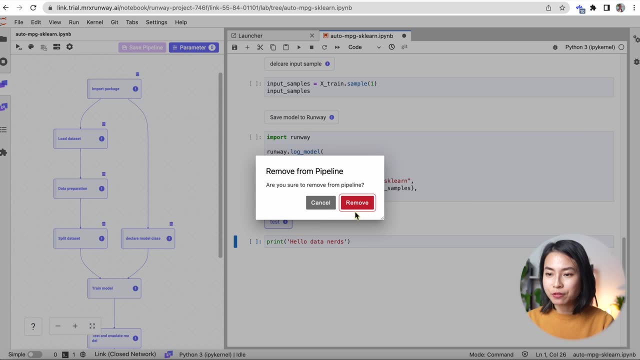 You can simply click on Add to the pipeline, Then enter the component name here and choose the parent component. So it is very, very simple. But let's remove this cell for now. So let me quickly walk you through this notebook to show you how this model is created. 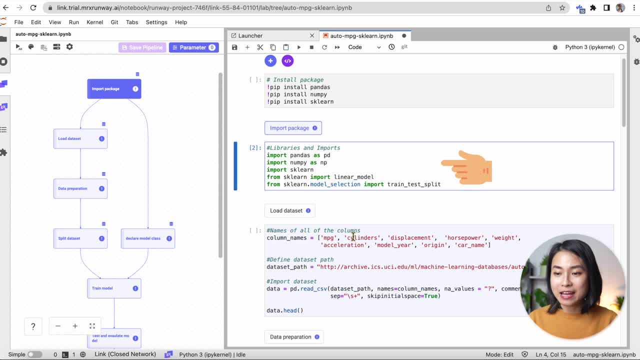 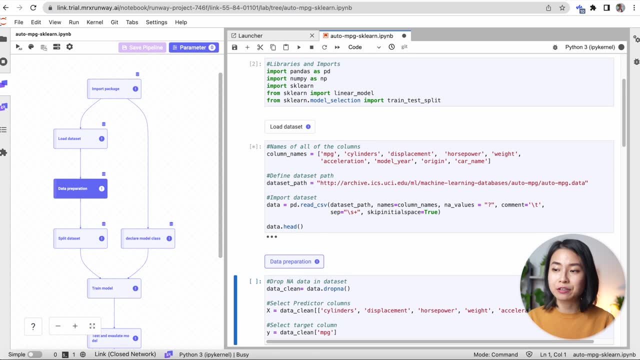 First we import some libraries, so pandas, numpy and scikit-learn, and some additional modules from scikit-learn. Then we import the auto-mpg dataset using this public data source. In practice it's most likely that we have to pull the data from the public data source. 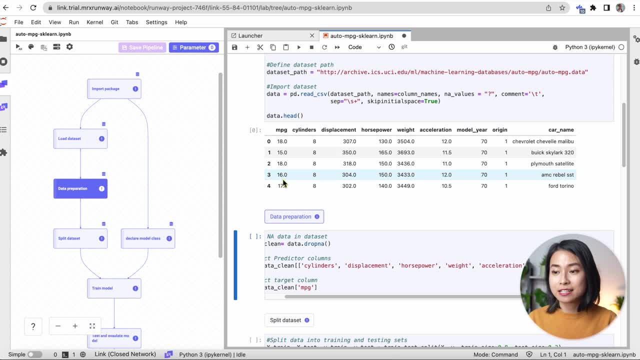 to get the data set from a database in your company And take a look at the dataset. We have the mpg column, which is the column we want to predict, and all the other attributes of a car that could be used as features, And then we can do some data preparation, removing some missing values. 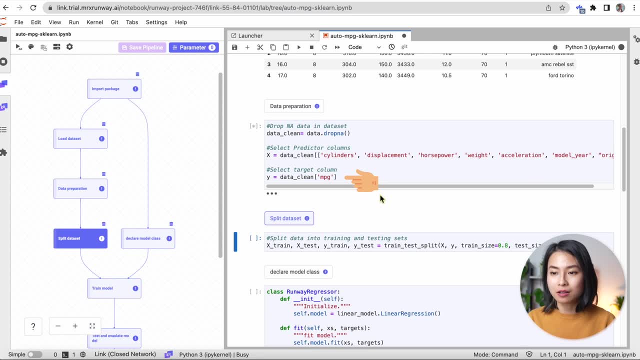 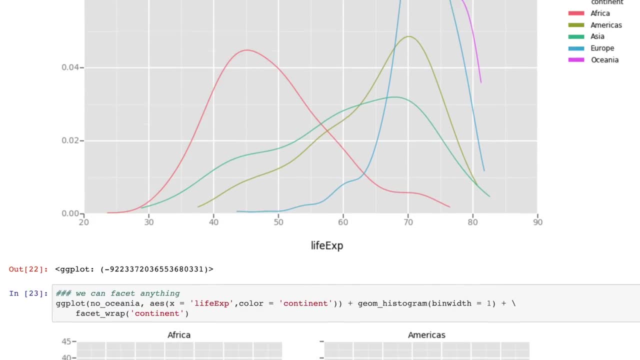 We also define the target column, which is the mpg column. This step is actually much more complex. in reality, We may need to do a lot of exploratory, data analysis and cleaning the data and transforming the data to get the data ready for modeling. 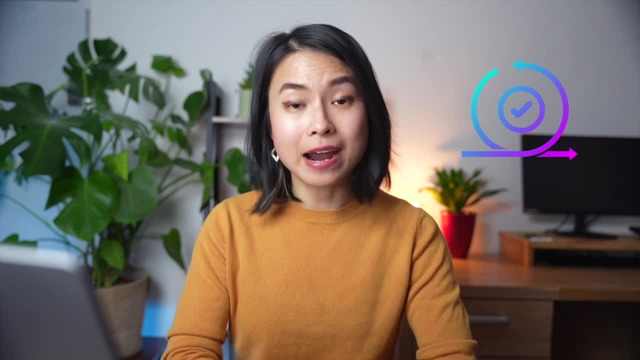 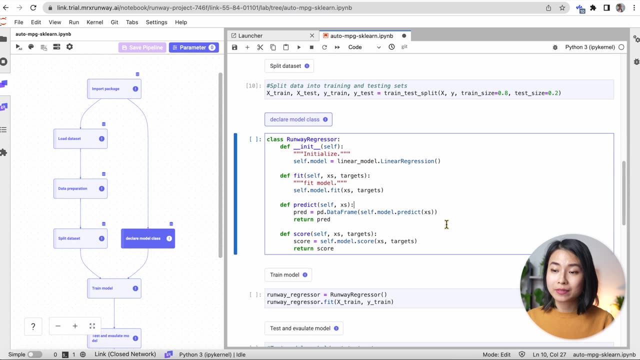 And we may also need to iterate several times to get it right, And after that we'll split the dataset into the training and the test set. Now we'll declare the runway regressor. Basically, this is a model object, where we define the model to be used and the functions. 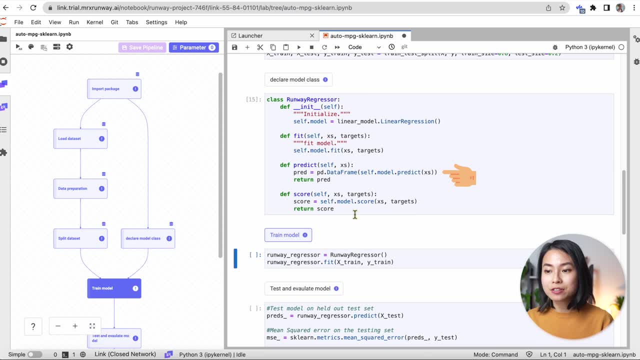 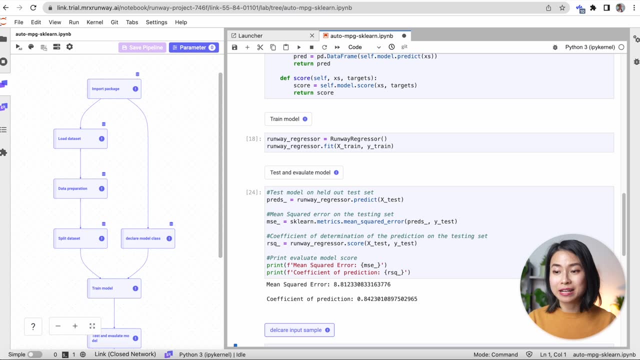 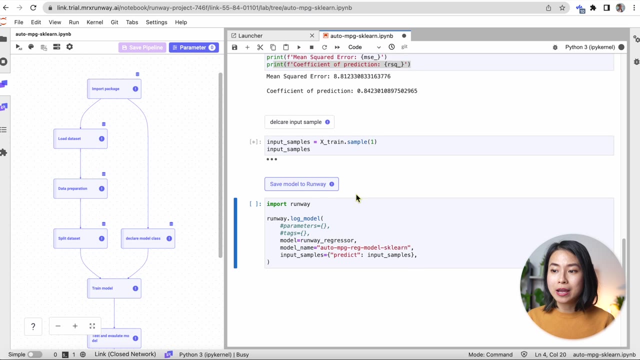 for fitting the model. as well as predicting output and scoring the model, Then we actually train the model using the training dataset and the training labels. After training the model, we test and evaluate. Next we'll declare an input sample by sampling a row in the training set. 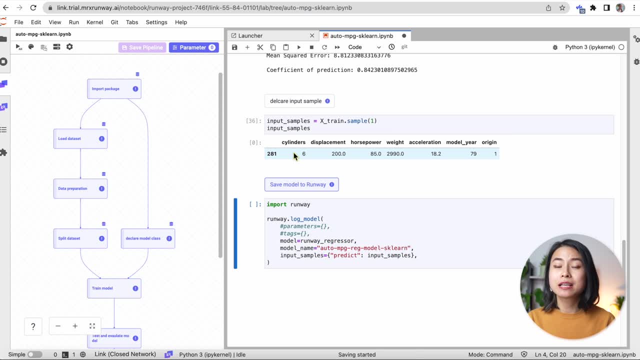 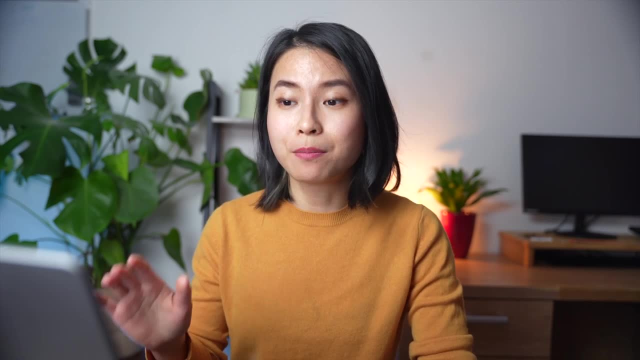 In production setting. it's often useful to provide model users with an input sample so that they know how the data should look like. So let's say everything is good and this is the final model that we have. We can now save the model to the runway platform. 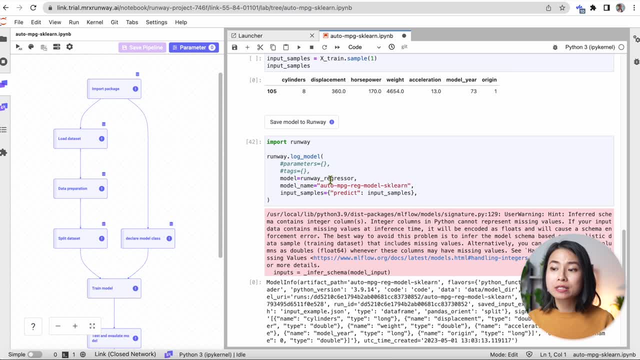 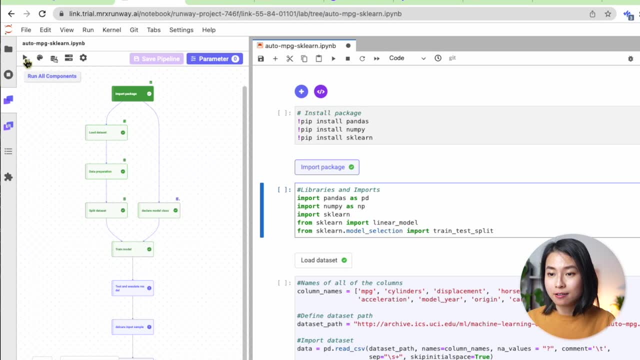 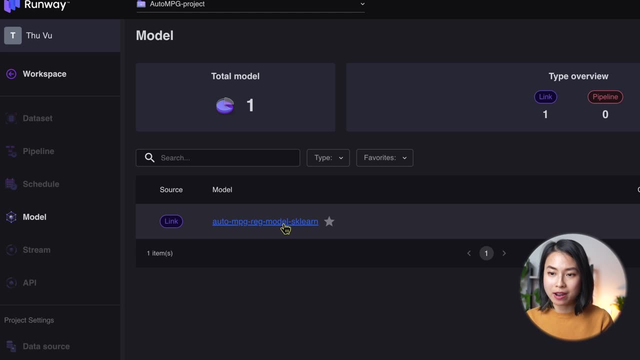 As you can see, all the cells in the notebook work correctly. We can also verify if this whole pipeline actually works By running all components. If we go back to the runway console, we can see that a new model called AutoMPGRegModelCycleLearn. 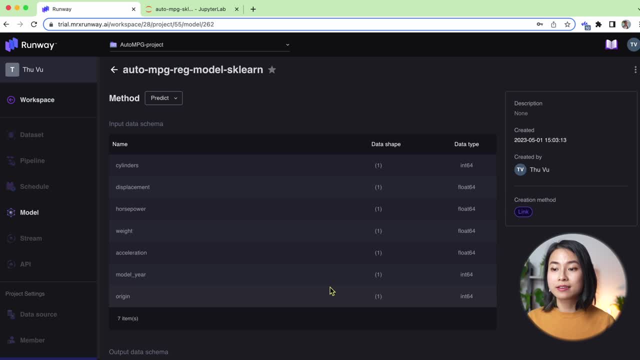 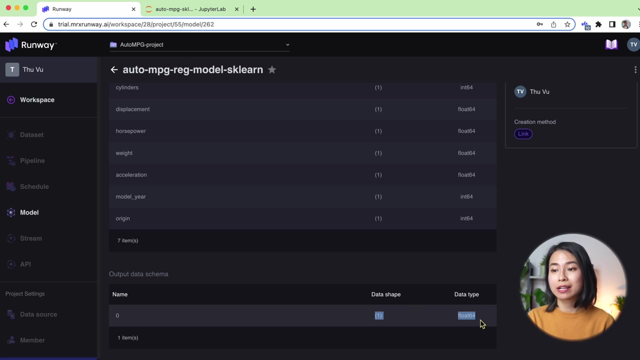 has been created. If we click on it, we can see all the methods of the model. So in this case, there's only one method, that is, predict, and the schema for the input data, including all the variable names, And we also have the output data schema, which is simply a numeric number, as the output. 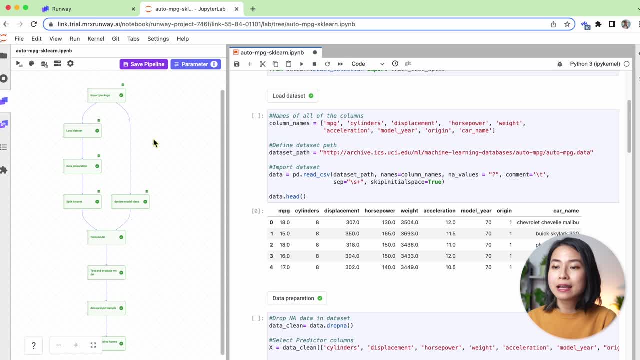 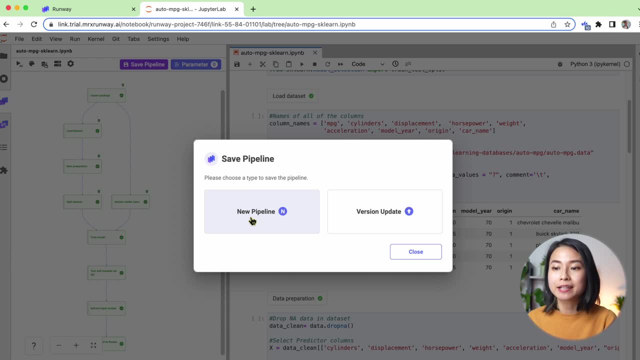 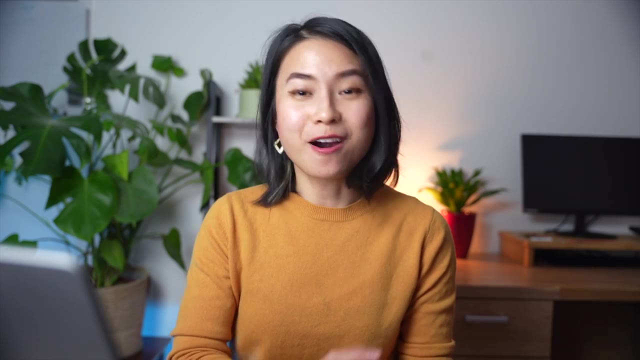 of the model prediction. Going back to development environment, we can click on save pipeline and click on new pipeline, because we don't have an existing pipeline yet, and name the pipeline as AutoMPGPipeline And click on save. Now here comes the exciting part. 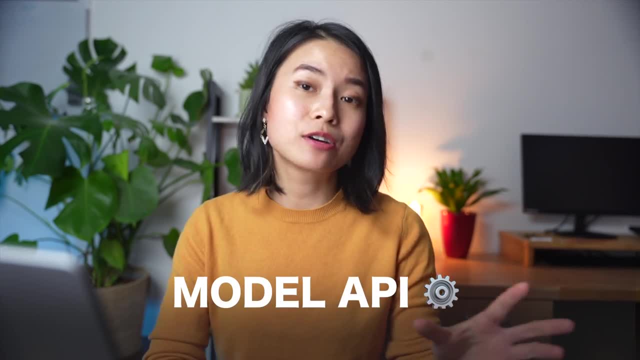 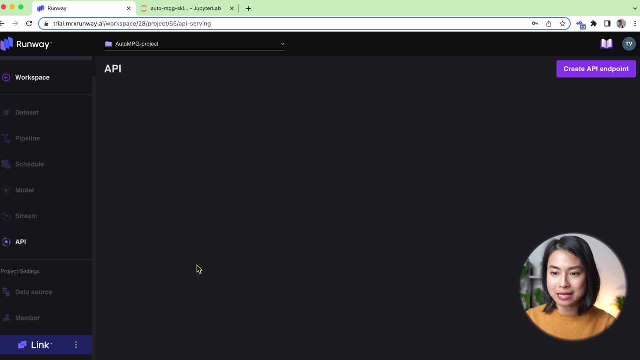 We'll create a model API so that other people can also access our model through the API to get the predictions on their data input. So let's go to the API menu And create an API endpoint over here And let's give our API a name. 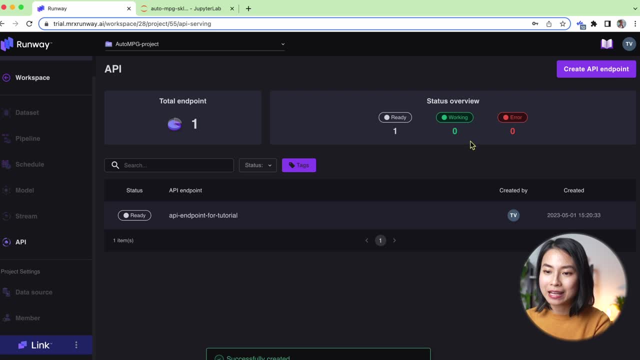 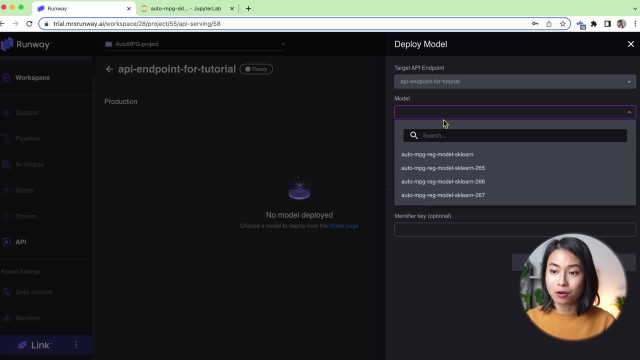 Let's say it's API endpoint for tutorial. We can now select the model that we want to attach to this API endpoint. So we'll select the model that we have just created And the model method is predict And the model instance type. I'll just use a micro, one gigabyte memory. 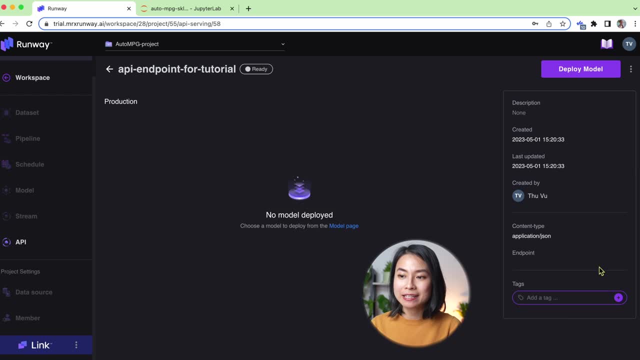 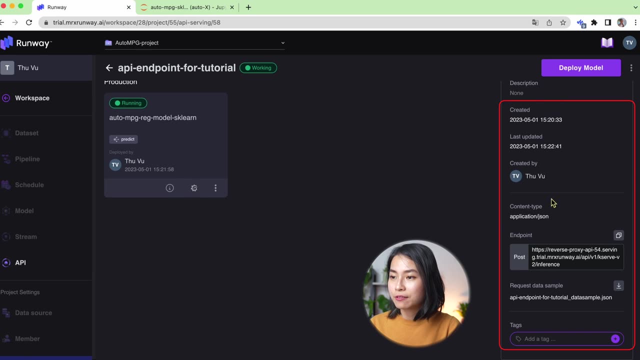 Let's click on deploy Now that we have the model API running. as you can see, the status is saved. The status is set to working. if the model service is running, On the right panel, you can see all the information of this API endpoint. 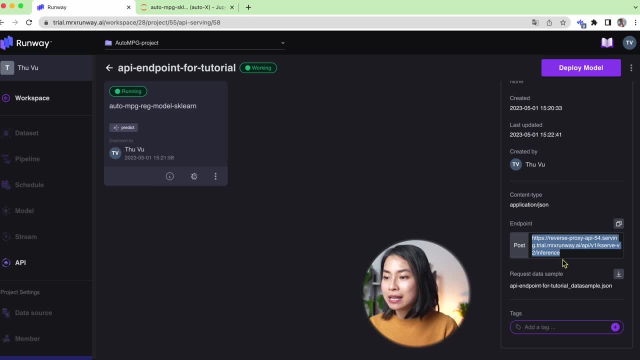 We have the content type, We have the API endpoint URL that we can share with model users, And we also have the data sample that we can download. Let's try to download this sample here and have a look at it. This is what the data sample looks like. 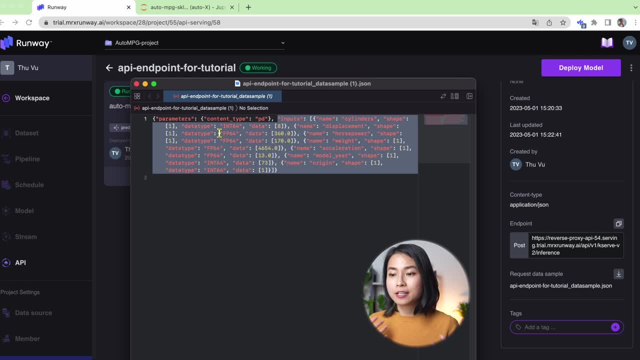 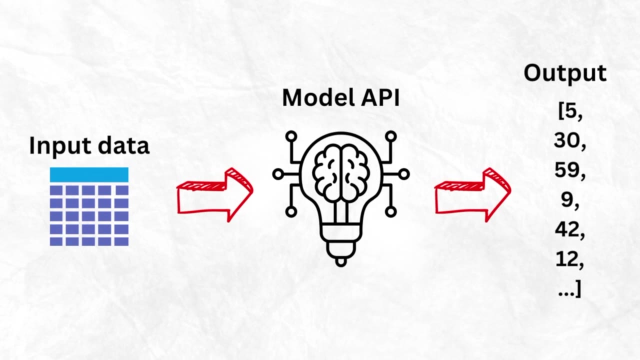 And this input part specifies all the variables, together with their data types and also their values, And this is based on the data sample that we created just now in the model pipeline. One way to interact with the model API is through the terminal. If you want to get predictions from the model for our own data input, we can use the client. 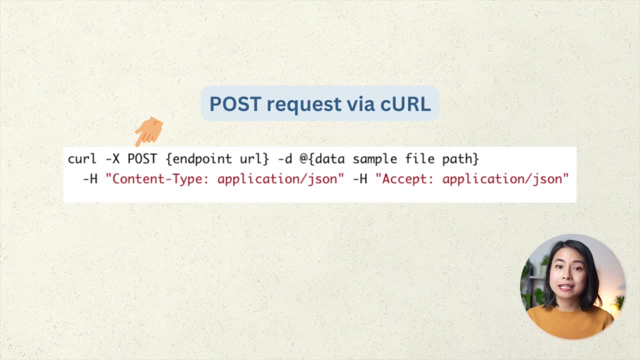 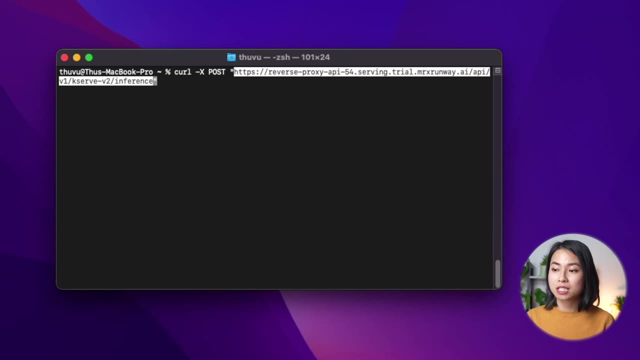 URL comment. using this format, We are basically creating a post request to the model API endpoint, which I'll copy from the platform over here, And we can specify the input data that we want to input to the model, which is the sample that we have here. 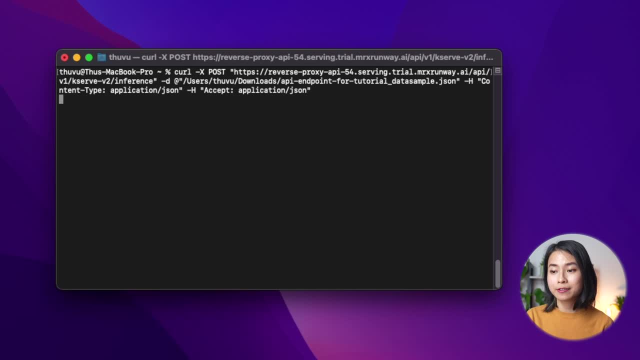 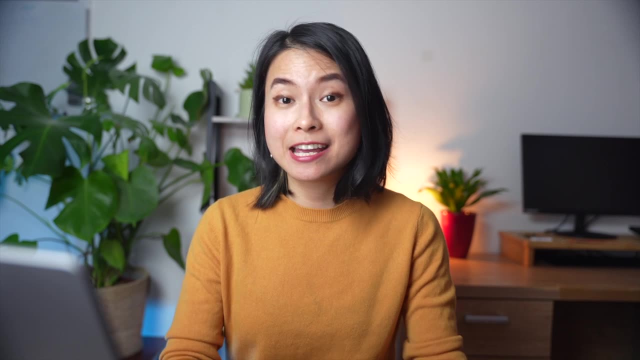 And some additional arguments over here. Let's now run this comment in the terminal And tada, we have the model predictions for our data input. As mentioned at the beginning of the video, after some time the model performance will almost certainly degrade. 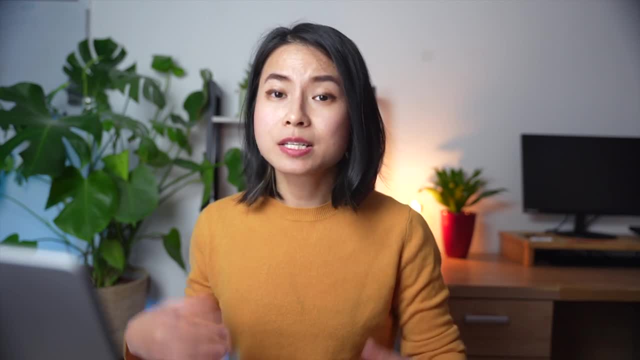 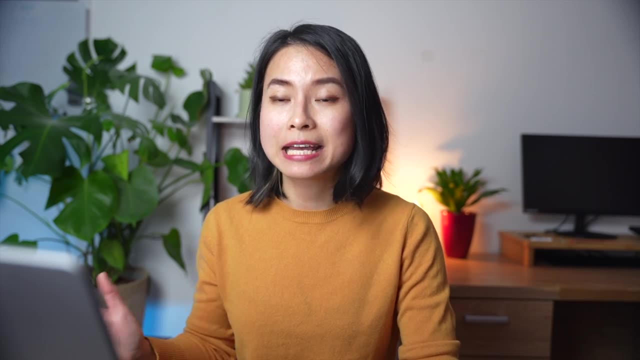 And this is when we need to retrain and redeploy the model. Suppose we have already done the retraining part by using new data or adjusting some things in the model code. We'll then navigate to the pipeline section on the runway construction And we can see that the model is already in the pipeline. 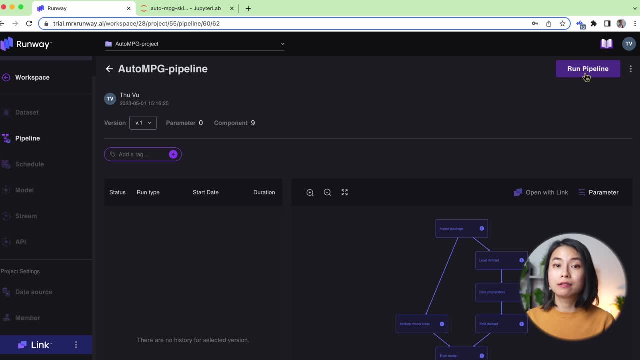 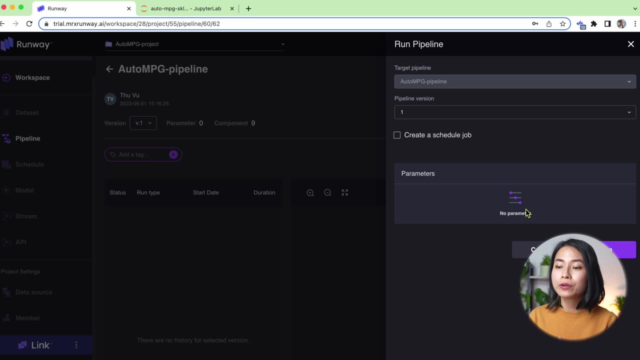 And we can see that the model is already in the pipeline. So click on the pipeline and then we can run the pipeline. If our model has some parameters, we can also input new parameters over here for our model. But in our case, having a simple linear regression model, we don't have any parameters. 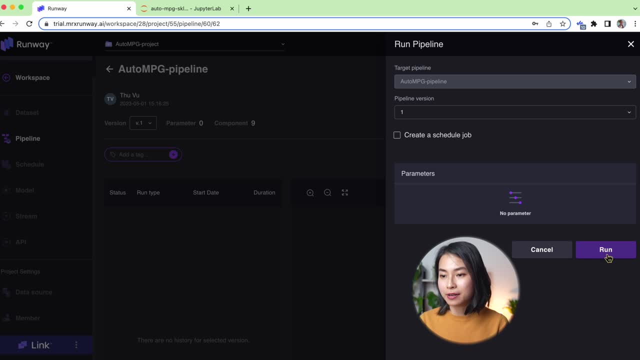 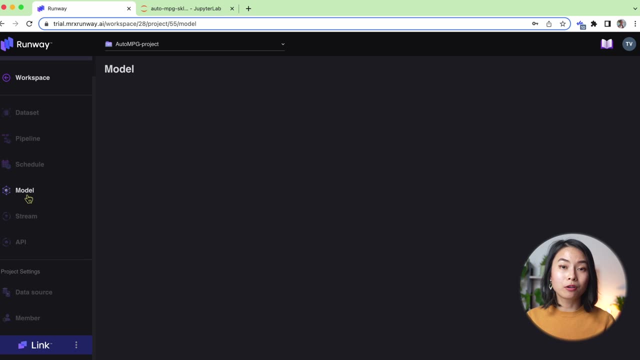 So let's just run the model by clicking on this run button And after the whole pipeline has been rerun, meaning that everything is now updated, we can go to the model page to redeploy the model. So if we click on the model, 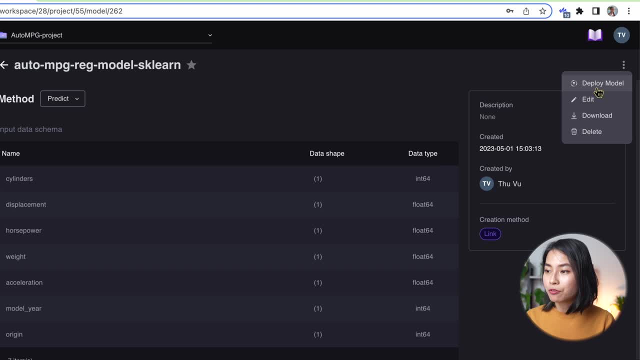 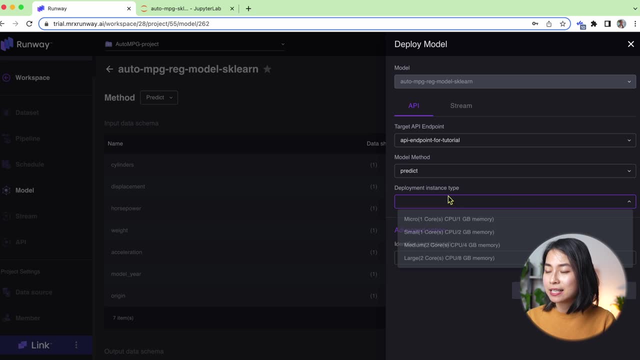 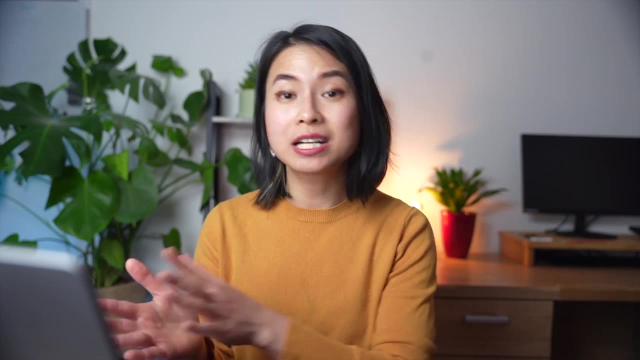 And click on the three dots over here, we can redeploy the model. We choose the target API endpoint for the model and select the methods, which is predict and the deployment instance type, And we can deploy the model again. This is basically how you retrain and redeploy the model on the runway platform. 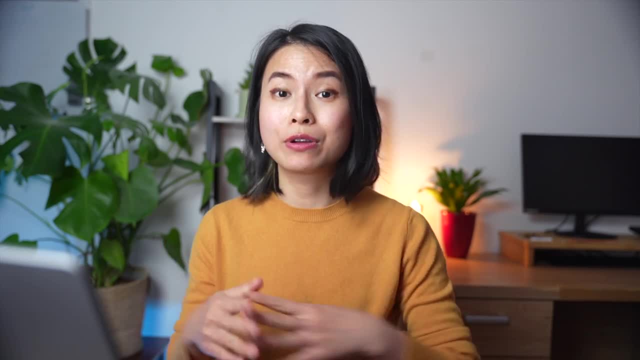 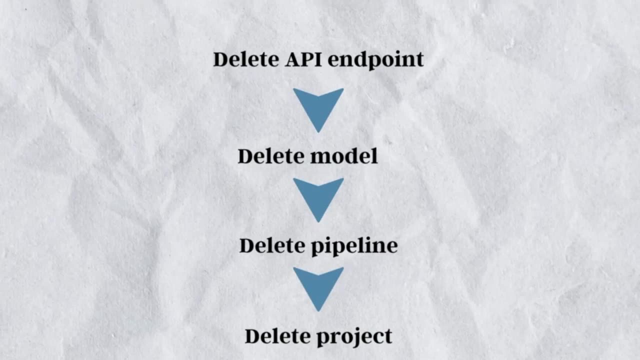 At some point in the future we may no longer use this model and we want to delete the model and the whole project to free up the resources. To do that, Let's first delete the API endpoint, and then the model and the pipeline and finally the 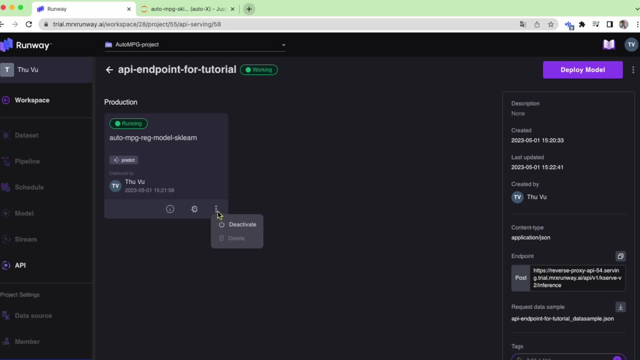 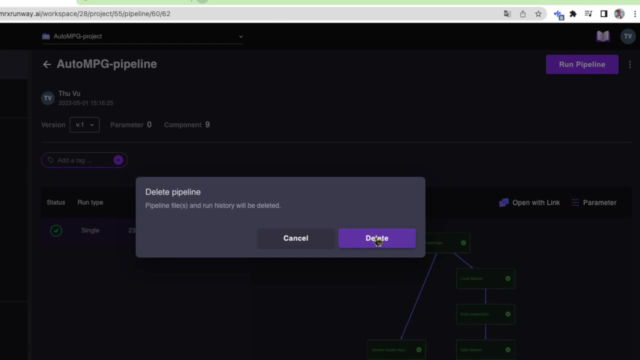 whole project. This is quite straightforward on the platform. We can easily deactivate or delete the API endpoints, the models or projects throughout the workflow with a single click. So I hope this demo gives you a better idea of how the model deployment process looks like. 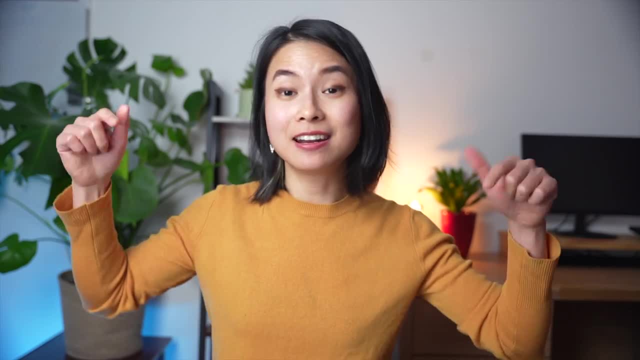 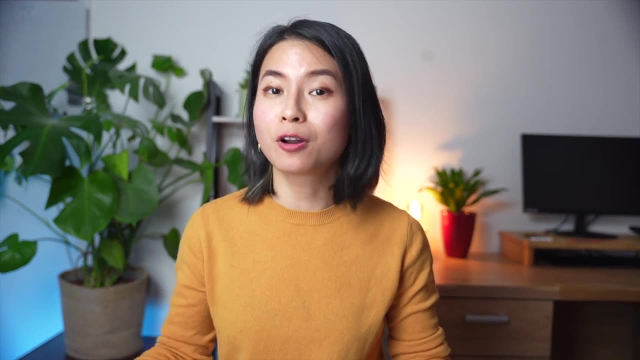 If you want to try out the runway platform to deploy your own model, check out the link in the description below and feel free to contact Makino Rocks for a free trial. And if you want to learn more about topics around model deployment and the practical